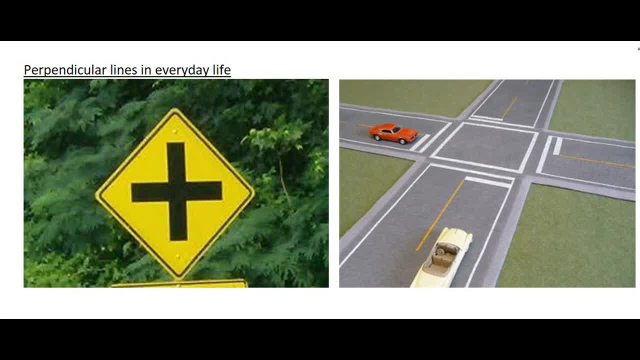 In this video we are going to look at perpendicular lines Now. perpendicular lines are exactly the opposite of parallel lines. So parallel lines have the same gradient, whereas perpendicular lines are completely opposite. The one line would go, for example, in this direction and the other line would go in the complete opposite direction. So here we can see some everyday life examples of 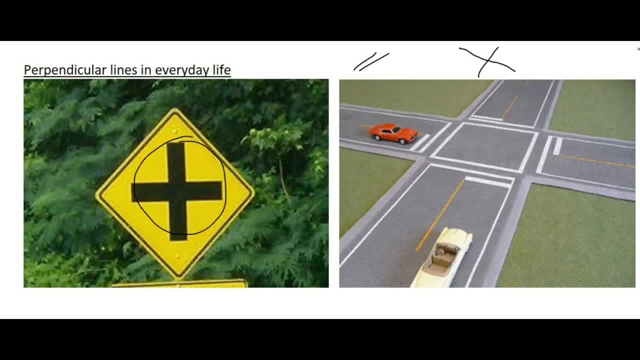 this signboard. Well, those two lines would be parallel because they are hitting each other at 90 degrees. They are going in the completely opposite directions. This four-way stop over here is also parallel, because I mean perpendicular, because these lines are hitting each other at 90. 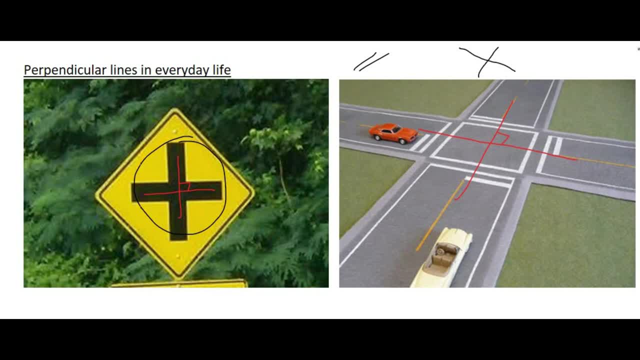 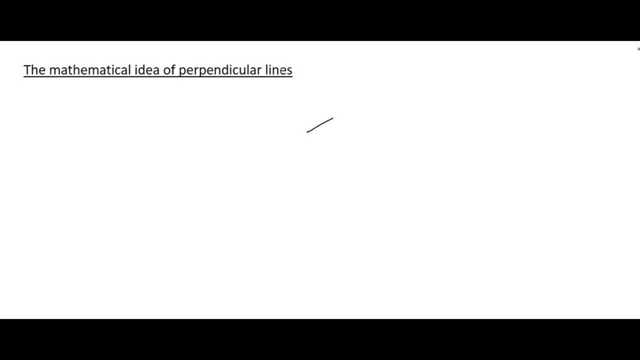 degrees. So perpendicular lines hit each other at 90 degrees. But what exactly does this mean mathematically? So when we looked at parallel lines, we said that parallel lines have the same gradient. So we said that parallel lines have the same gradient. So we said that. 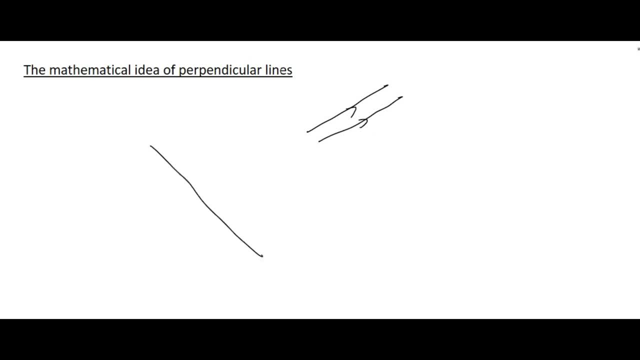 parallel lines have the same gradient. However, perpendicular lines are completely opposite to each other and they always hit at 90 degrees. It's quite interesting, but what this means mathematically is that if you multiply the two gradients together, if the lines are perpendicular- 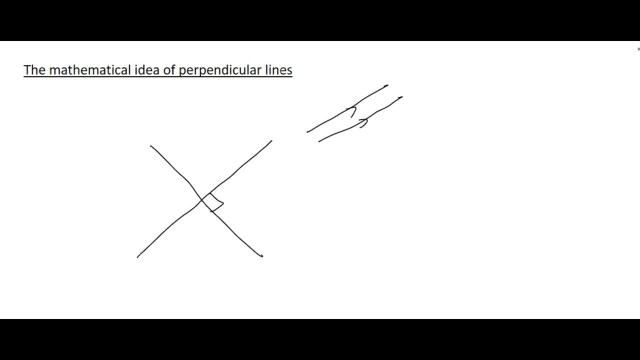 your answer should always be negative one. So we can say that the gradient of line one times by the gradient of line two will give you an answer. So the following calls a gradient of: if that happens, then the lines are perpendicular. Let's see how this works. So let's say the gradient of this line is two. now love. 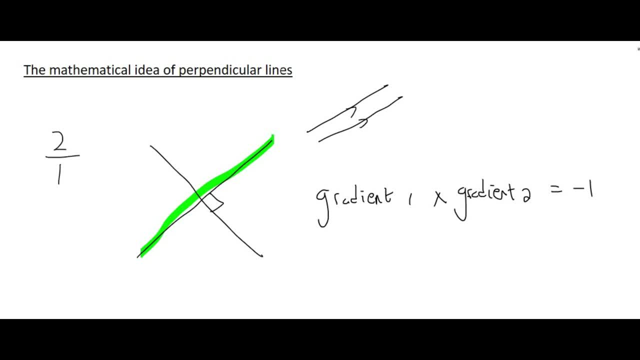 the same as 2 over 1, right? So what is the complete opposite of that? Well, the complete opposite of that is this: You have to switch the number over, So it will be one over two, and then change the sign, And so if it's a positive, it will change it to a negative. so 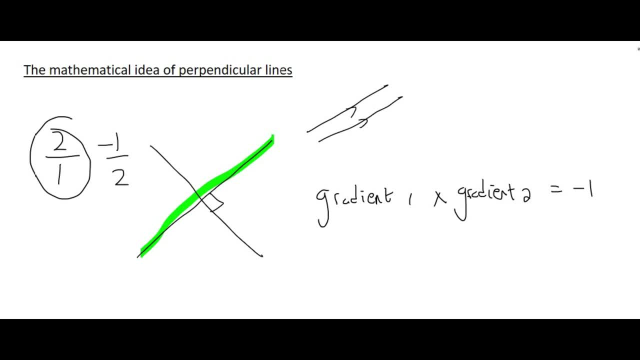 So we'll change this to a negative. If we now had to multiply these two lines together- or, sorry, if we had to multiply the two gradients together, what you would see is that the 2s would cancel, the 1s would cancel and you'd just be left with minus. 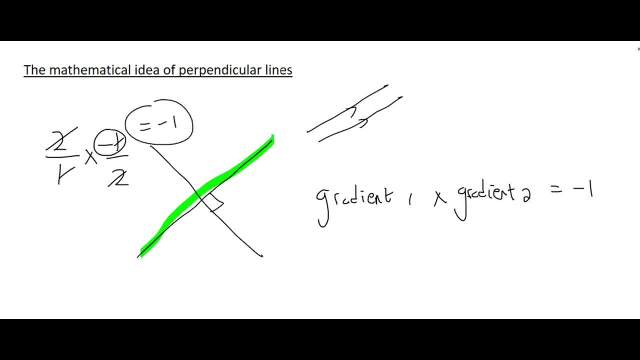 So you'd be left with an answer of minus 1.. So whenever the gradients of two lines, when you multiply them together, if that gives you an answer of minus 1, then the lines are perpendicular. So let's try a few examples. 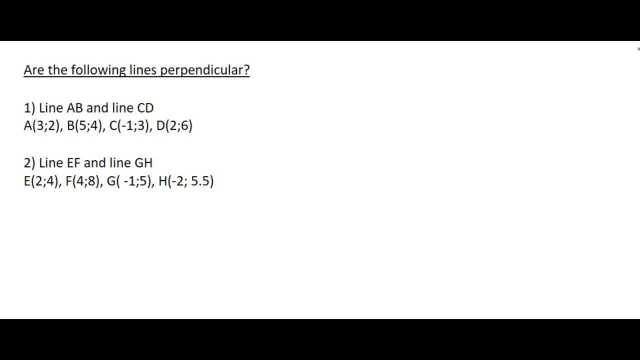 The question asks us: are the two lines perpendicular? So here we have line AB and we have line CD. So let's go work out the gradient of each of them and then see if their lines are going to be, or if their gradients are going to be, perpendicular. 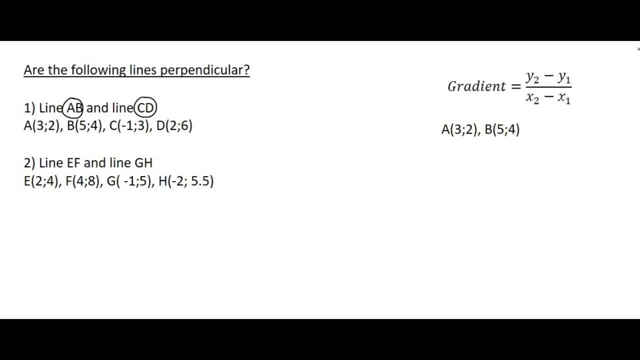 So let's take a look at line AB first. Well, if we use the gradient formula, I'm going to call point A number 2 and point B number 1.. That's just my choice. It doesn't have to be your choice. 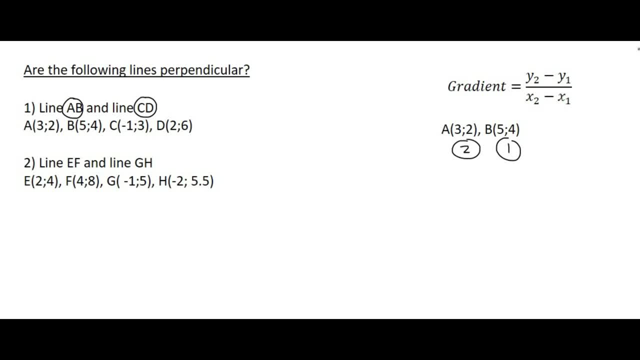 So I'm going to call point A, number 2, and point B, number 1.. So you can choose it the other way around, but you'll still get the same answer. So if we use the formula, it says that we should take the y value of point number 2.. 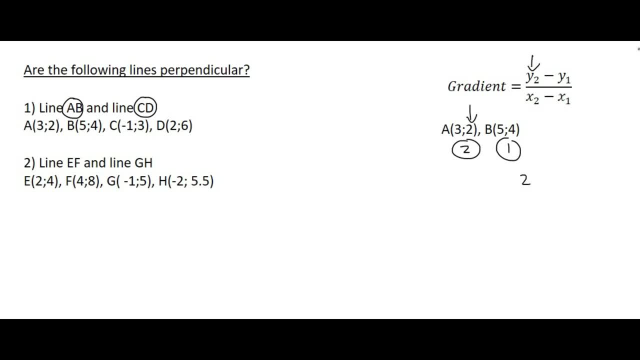 Well, the y value of point number 2 is 2.. Then we should use a minus, And the y value of point number 1 is a 4.. Then we go to the x value of point number 2, which is 3.. 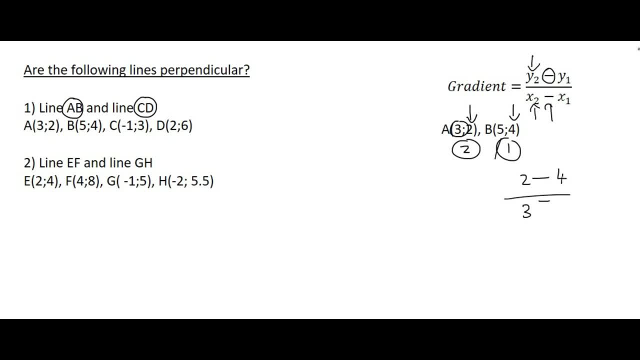 Then it says minus, And then we take the x value of point number 1, which is a 5. And if you had to go type all of this in on the calculator, you're going to get an answer of minus 1.. 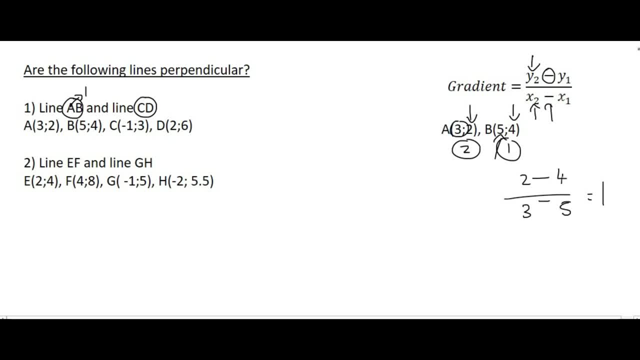 And you're going to get an answer of 1.. So the gradient of A- B is 1.. So now we can move on to the gradient of C- D, And so I'm going to call C point number 2 and D point number 1.. 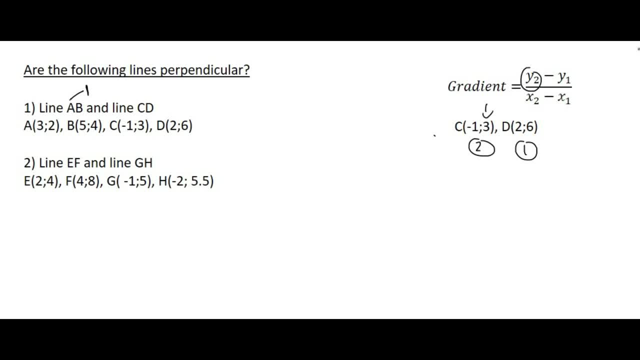 And so the formula says I should start with the y value of point number 2,, which is a 3, minus, Then the y value of point number 1,, which is a 6. Then it's the x value of point number 2,, which is minus 1.. 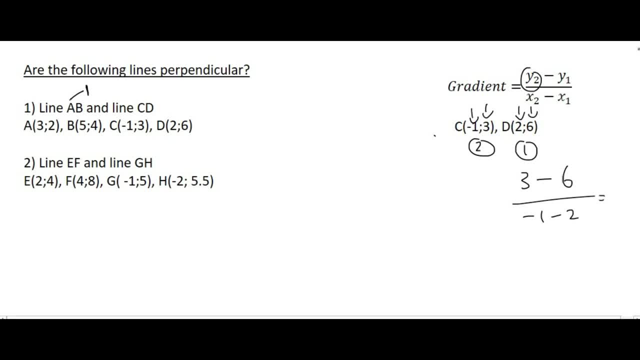 And then the x value of point number 1, which is 2.. And if I had to go work this out, I would end up with 1.. And so line C D's gradient is 1.. And so these two lines are not going to be perpendicular. 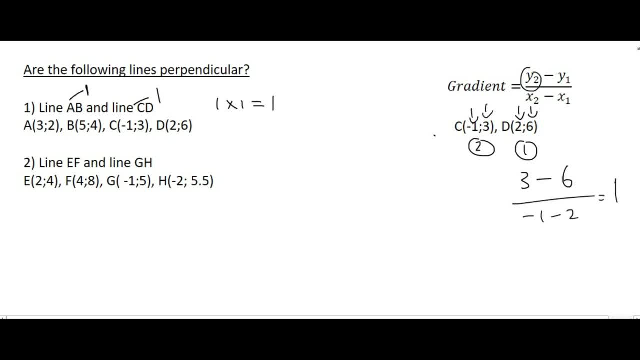 because if you multiply 1 with 1,, you are not going to get minus 1, but you're rather going to get 1.. So, in fact, because these two gradients are the same, they are actually called parallel. Well done to any of those of you who remember that. 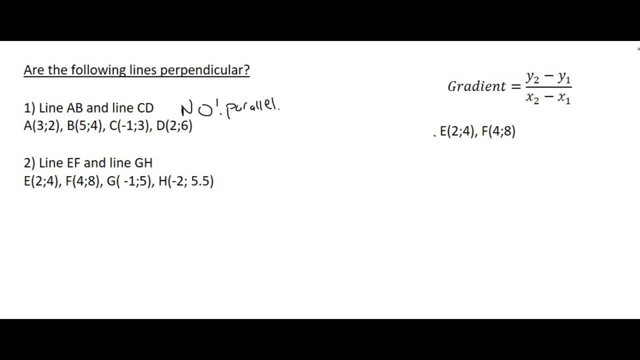 If the gradients are the same, it's parallel. Moving on to number 3. Number 3.. Number 3., Number 2.. Let's work out the gradient of EF. So I'm going to call this point number 2 and call this point number 1..